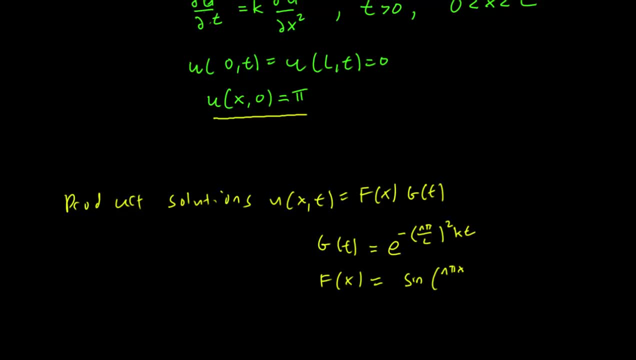 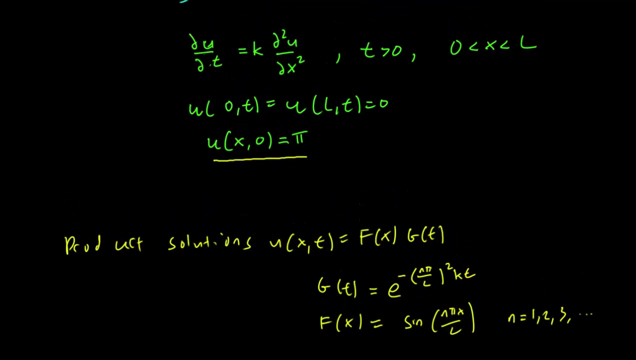 to sine n, pi, x over L for n. 1,, 2,, 3, and so on, All the positive integers. Again, recall that by plugging in the product solution- uxt equals fxgt- into the heat equation formula, We reduce the differential. 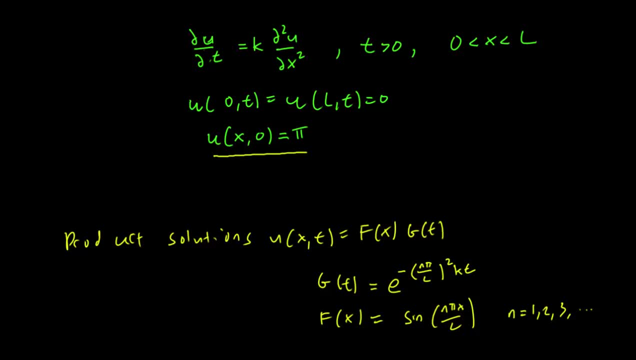 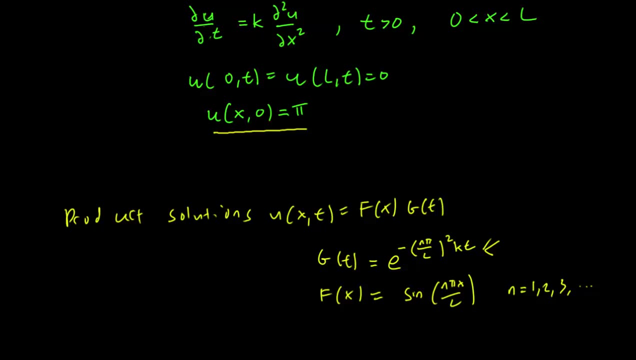 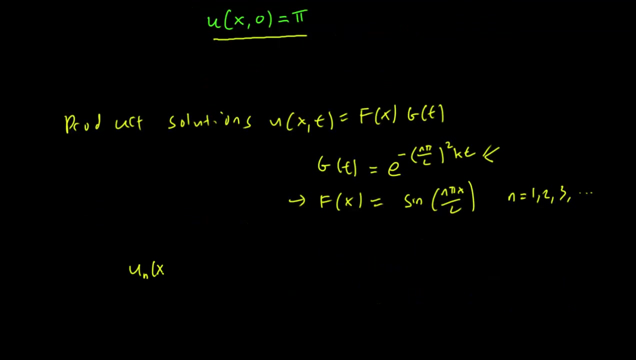 equation for the heat equation into two equations: one that we can solve using separation of variables, which is the g solution, and one which we solve using the eigenvalue method, which is the f solution. So the product solutions are of the form: u. nxt equals e minus n, pi. 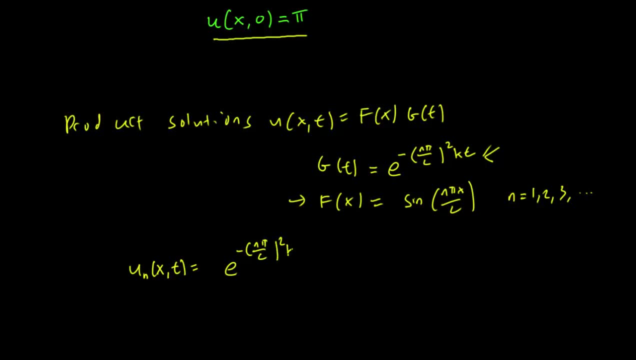 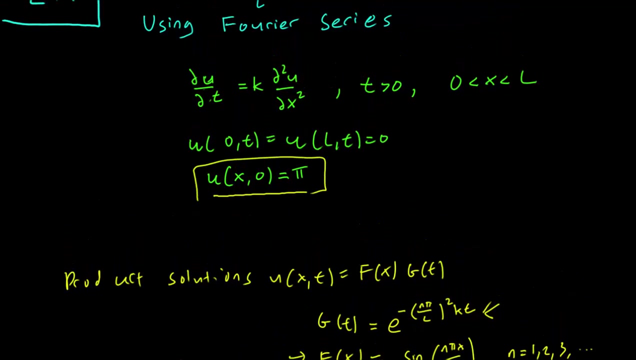 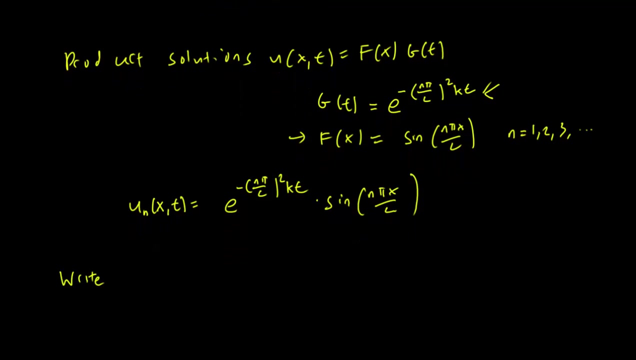 over l squared kt times sine n pi x over l. So we need to figure out how we can get the initial condition: u equals pi. We have to figure out how to write pi as a sum of sines, of the form sine n, pi x over. 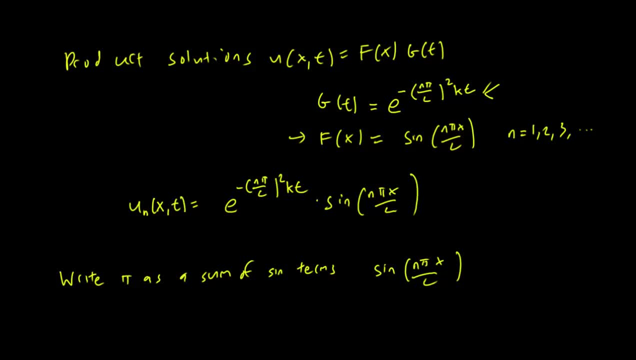 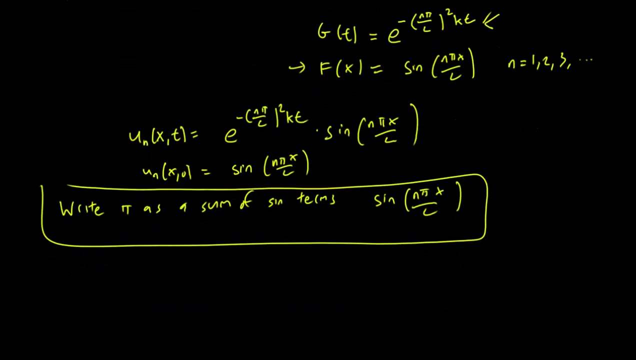 l because, if you may recall, taking initial conditions, setting t equals zero will turn these product solutions into sine terms of the form sine n, pi x over l. So we need to use the Fourier's theorem here. So pi is equal to a sum, n equals zero to infinity. bn sine n, pi x over l. This is by: 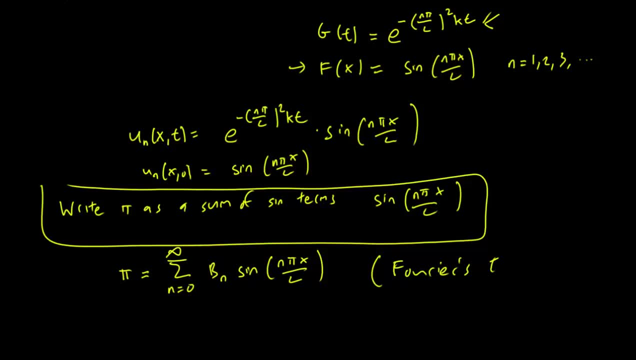 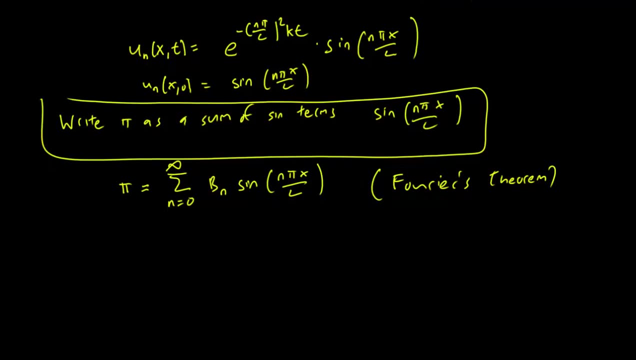 Fourier's theorem. It says that any function can be written in this form. And now we just need to find out what pi is, What the bn are, and from the Fourier's theorem video we know that we just have to find b. m is equal to two over l times the integral from zero to l of pi sine n, pi x over l dx. 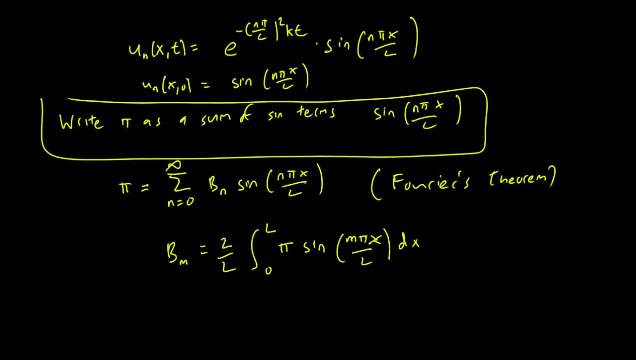 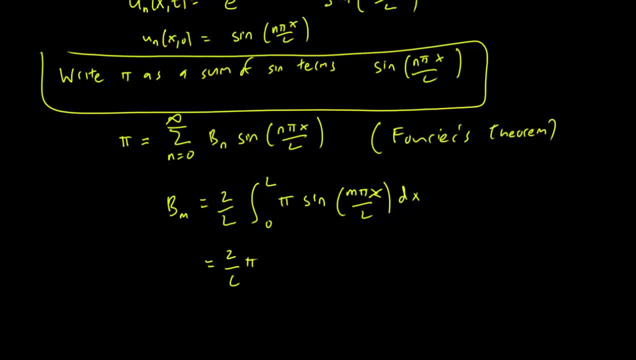 of the integral, of the integral of zero to l is of pi sine n pi x over l dx, then we can- I can- pull the pi out there because it's constant and the integral of sine m pi LX is going to be minus cosine m pi LX times L over m pi, going from x equals 0 to x equals L. 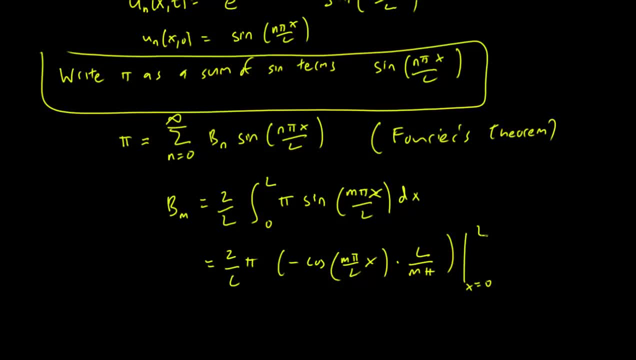 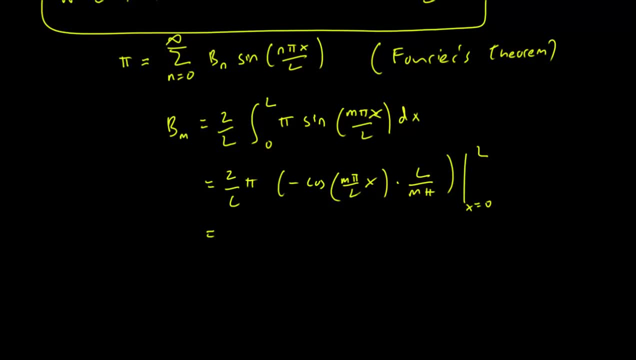 because those were our boundary conditions for the original integral. We can then simplify all the constants and we just end up with 2 over m, The pi's cancel out, the L's cancel out, and we just have 2 over m over there and we 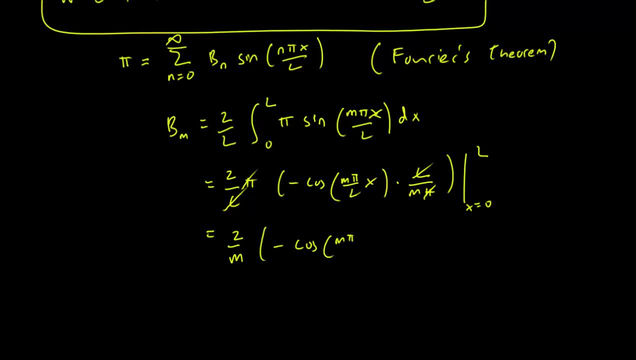 just have minus cosine m pi, X over L. going from x equals 0 to L. This is of course just going to be 2 over L, minus cosine m? pi, because we're plugging in L here. so we just have m? pi and plus 1, because cosine of 0 is 1.. 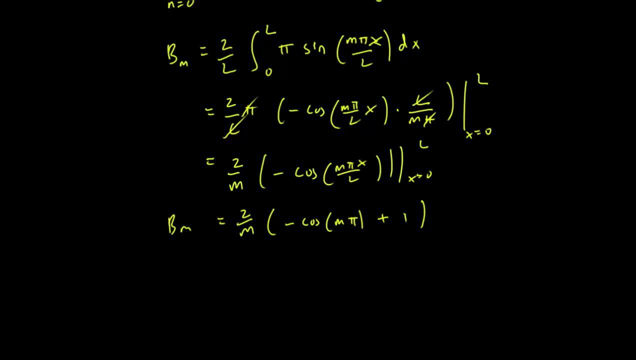 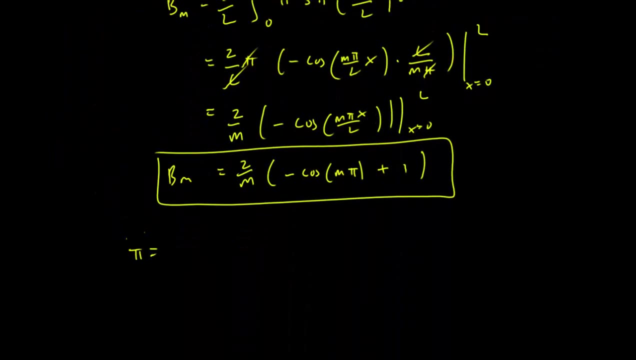 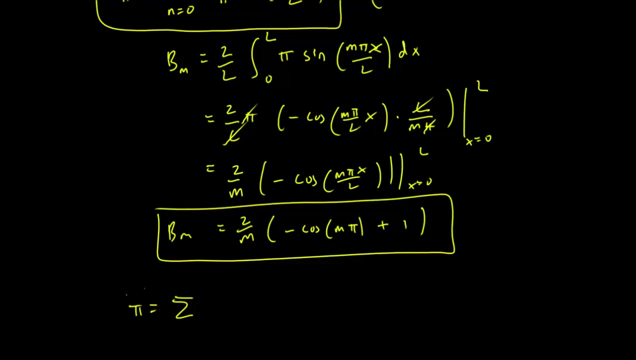 That is our value for Bm, if you may recall, And now all you have to do is to plug it back in. the Fourier theorem, Pi is equal to the sub-competitor sum. we know that bn is this term. It's going to be from: m equals 1 to infinity, 2 over m minus. 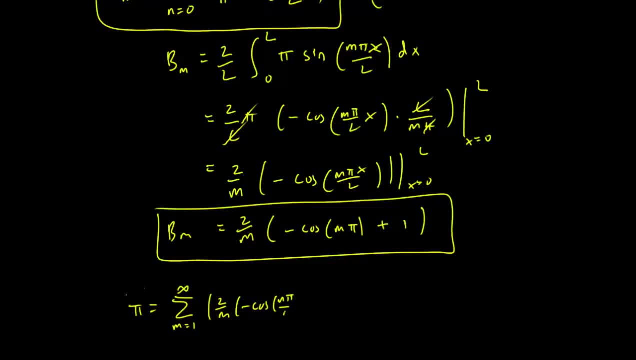 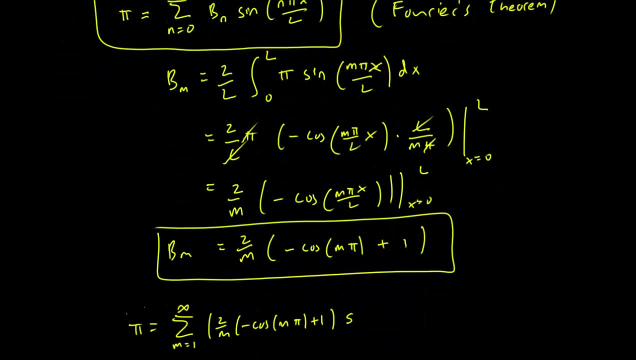 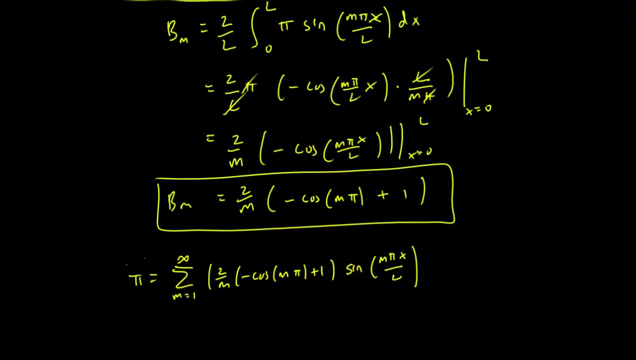 cosine m pi over l. sorry, it's just m pi plus 1 multiplied by sine m pi x over l. Actually, let's just change it back to n, since that's what I wrote down in the first place. So let's just replace all the m's with n's, just to make it. 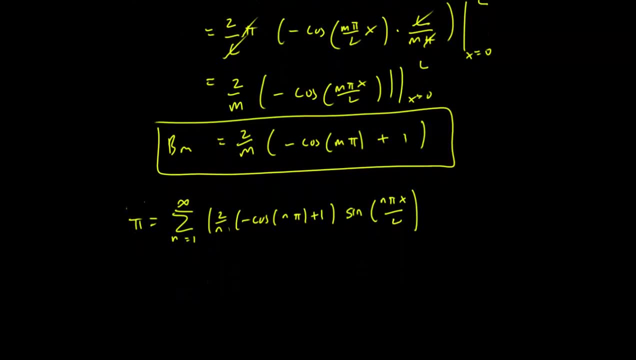 consistent. it doesn't matter what letter you use. Let's simplify this expression a little bit. it looks a bit nasty, But you can note that cosine of n? pi is 1 for n even and cosine of n? pi is minus 1 for n odd. 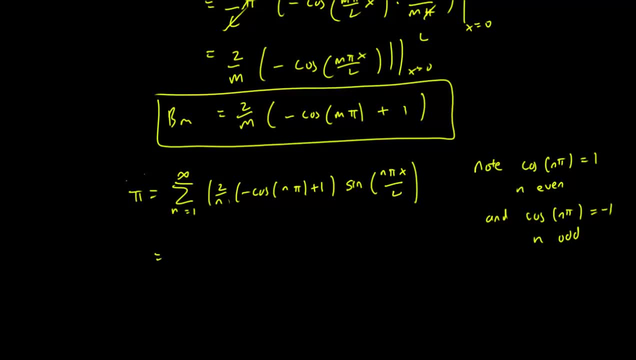 This means that if n is even, we just get minus 1 plus 1 here, and this entire term disappears. When n is odd, this is just a 2. So we can ignore all the cases when n is even. so we can say we're just summing: the case of n equals. 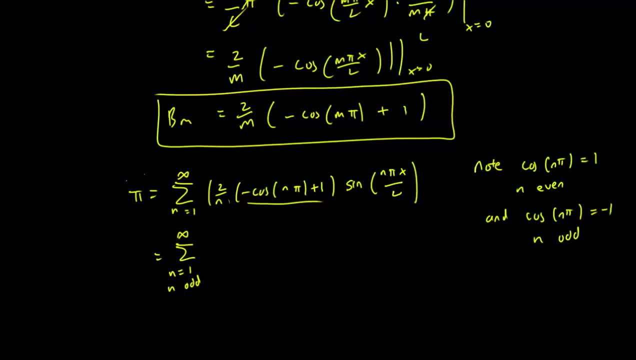 1 to infinity of n odd. To sum the case, from n equals 1 to infinity, we've n odd, and when n odd, this is a 2, and the sine remains. and when n is, even the term disappears. So we have this, and this of course simplifies. to sum of m. 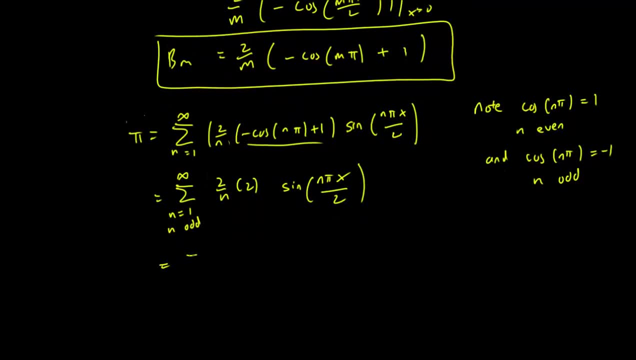 equals 1 times n odd. So that's the final definition of this expression. I hope you found it helpful And thanks for watching. equals 1 n odd, 4 over n sine n, pi x over L. 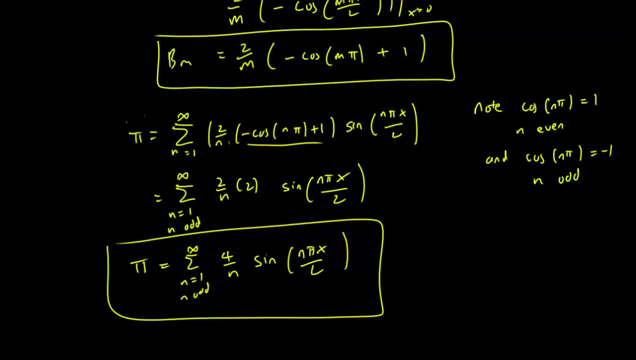 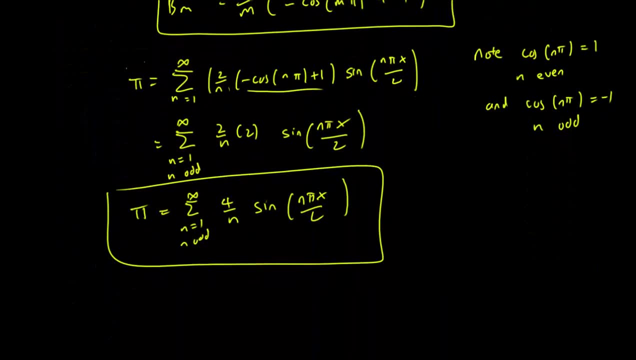 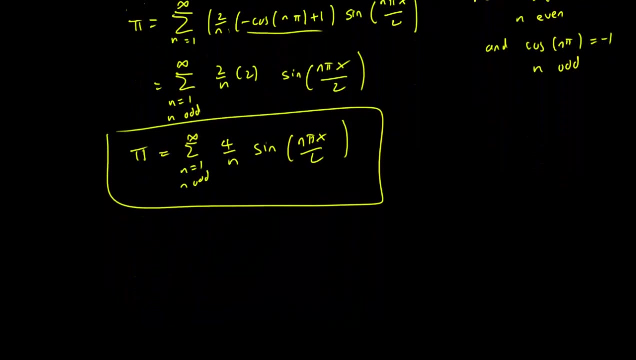 That's our expression for pi. So we wrote down our initial condition over here in terms of sum of sines, just as we required, And now it's not too difficult to figure out what our general solution should be. So if you remember our general solution, 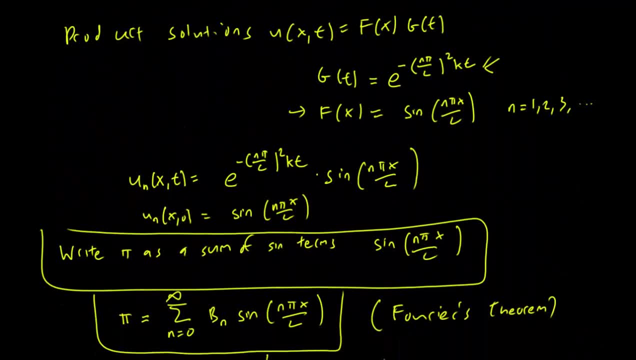 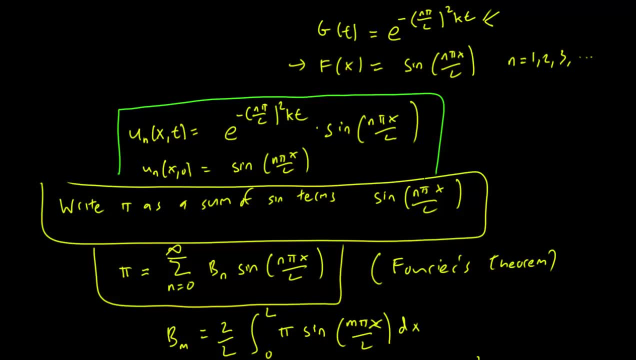 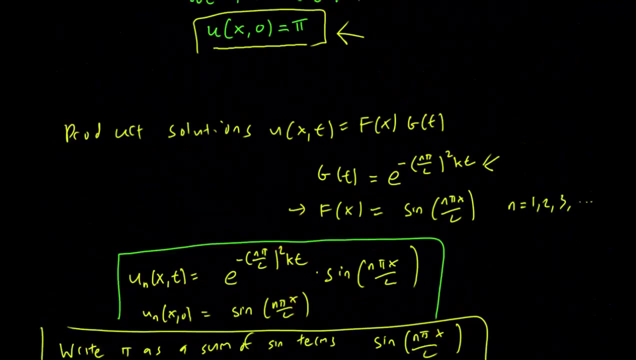 will be written in as a sum of product solutions. Let's go back to product solutions. So these are the product solutions over here, And we want to replace all the sine terms with the un terms. So we have here: n equals 1.. 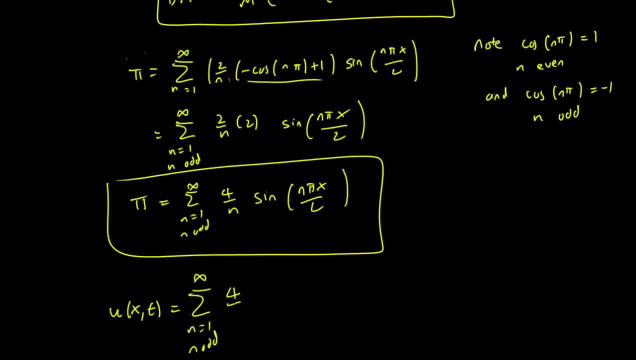 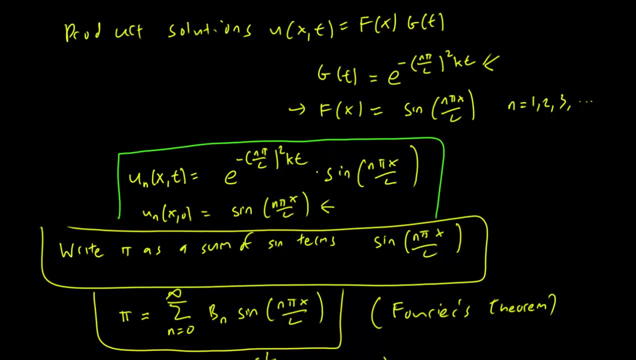 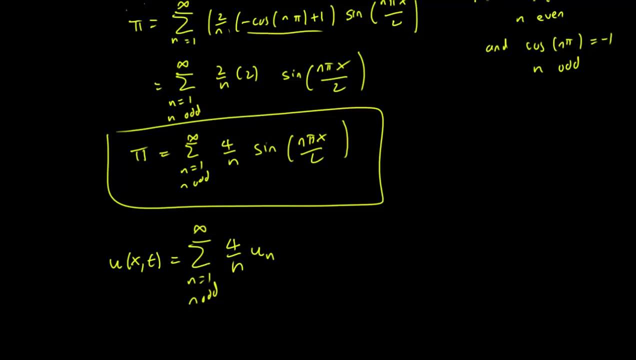 N odd again, infinity 4 over n instead of sine n pi x over L, Because the initial condition of the product solution is sine n pi x over L. So we replace this with un And this is exactly our solution to the original problem. 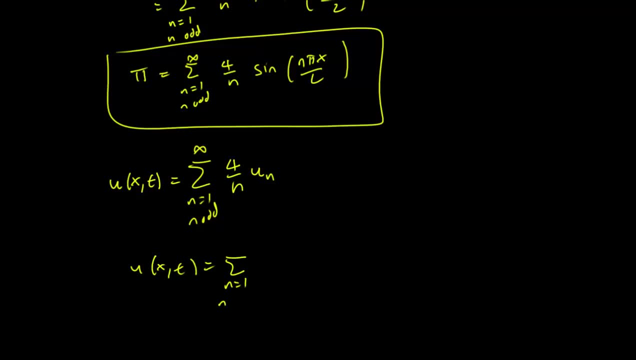 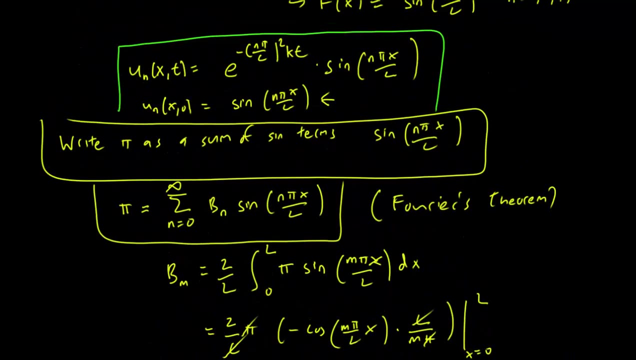 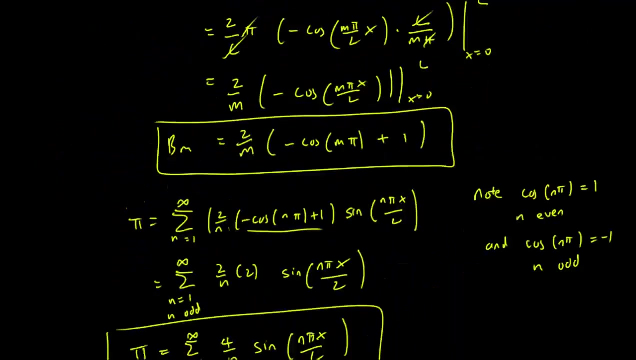 Let's just write out the un So n over 1, n odd infinity 4 over n times un u n is of course just going to be e minus n pi over L, squared kt times sine n pi x over L. And if we look at that,